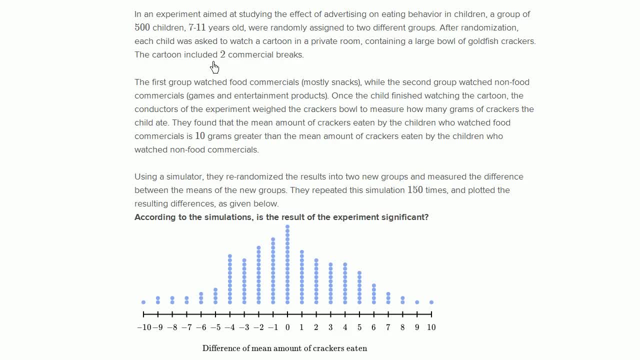 a large bowl of Goldfish crackers. The cartoon included two commercial breaks. The first group watched food commercials, mostly snacks- while the second group watched non-food commercials- games and entertainment products. Once the child finished watching the cartoon, the conductors of the experiment weighed the cracker bowls to measure how many grams of crackers the 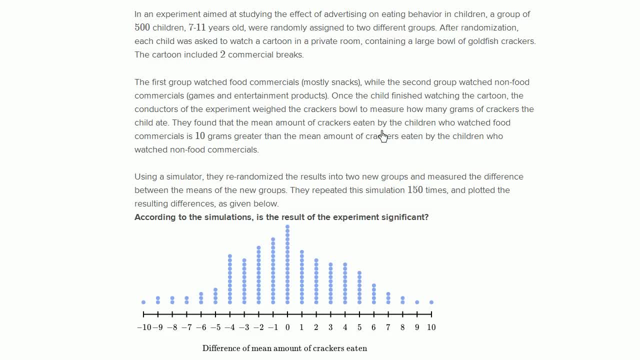 child ate. They found that the mean amount of crackers eaten by the children who watched food commercials is 10 grams greater than the mean amount of crackers eaten by the children who watched non-food commercials. So let's just think about what happens up to this point. So they took 500 children. 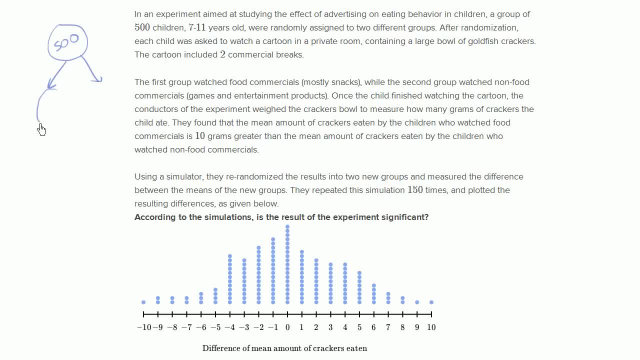 and then they randomly assigned a group of 500 children to watch a cartoon in a private room. They assigned them to two different groups. So you have group 1 over here and you have group 2.. So let's say that this right over here is the first group, The first. 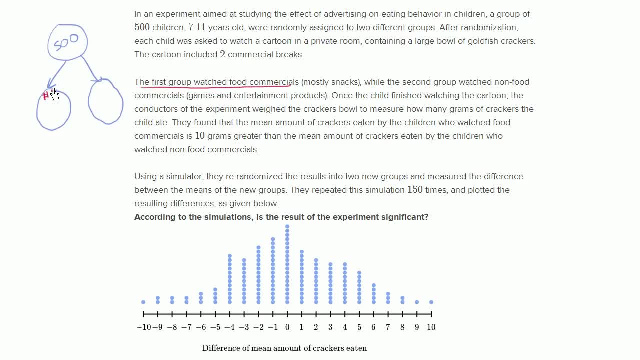 group watched food commercials. So this is group number 1.. So they watched food commercials. We could call this the treatment group. We're trying to see what's the effect of watching food commercials. And then they tell us the second group watched non-food commercials. 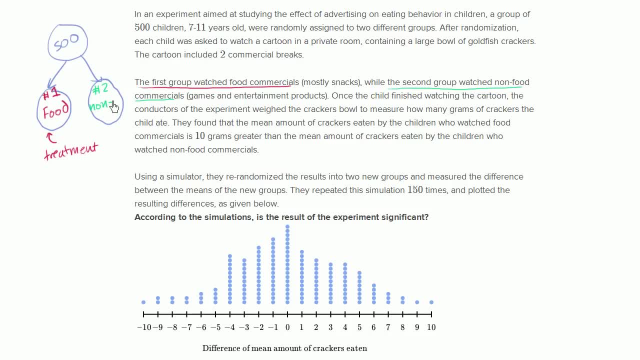 So this is the control group. So number 2, this is non-food commercials. So this is the control right over here. Once the child finished watching the cartoon, for each child they weighed how much of the crackers they ate And then they took the mean of it and they found that the mean here. 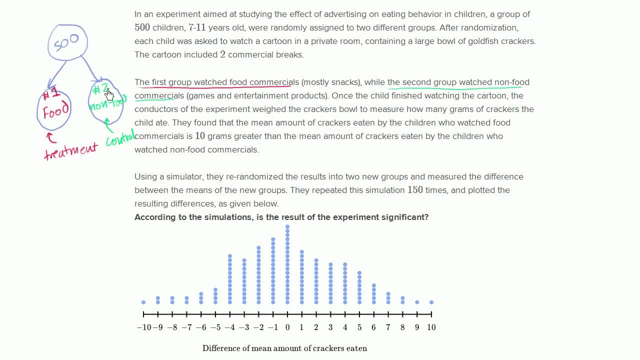 that the kids ate 10 grams greater on average than this group right over here, which, just looking at that data, makes you believe that OK. well, something maybe happened over here, that maybe the treatment from watching the food commercials made the students eat more. 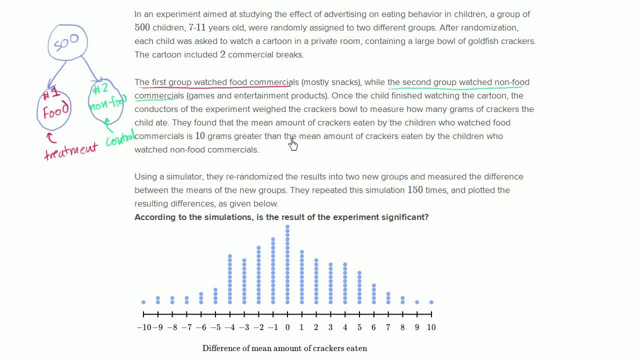 of the goldfish crackers. But the question that you always have to ask yourself in a situation like this: well, isn't there some probability that this would have happened by chance? that even if you didn't make them watch the commercials, If these were just? 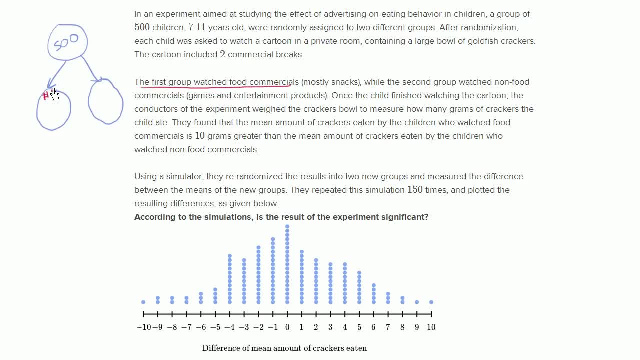 group watched food commercials. So this is group number 1.. So they watched food commercials. We could call this the treatment group. We're trying to see what's the effect of watching food commercials. And then they tell us the second group watched non-food commercials. 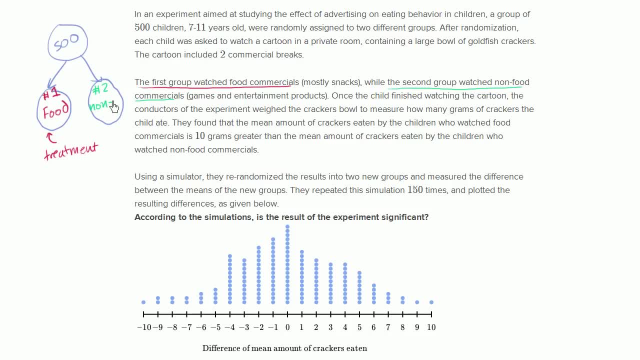 So this is the control group. So number 2, this is non-food commercials. So this is the control right over here. Once the child finished watching the cartoon, for each child they weighed how much of the crackers they ate And then they took the mean of it and they found that the mean here. 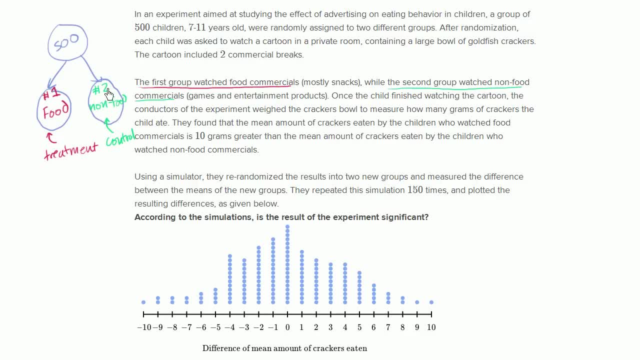 that the kids ate 10 grams greater on average than this group right over here, which, just looking at that data, makes you believe that OK. well, something maybe happened over here, that maybe the treatment from watching the food commercials made the students eat more. 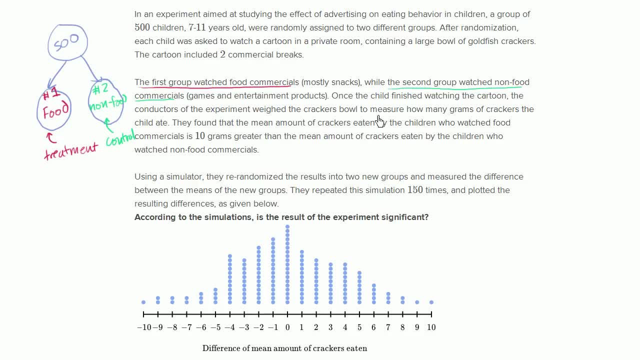 of the goldfish crackers. But the question that you always have to ask yourself in a situation like this: well, isn't there some probability that this would've happened by chance, That even if you didn't make them watch the commercials, if these were just? 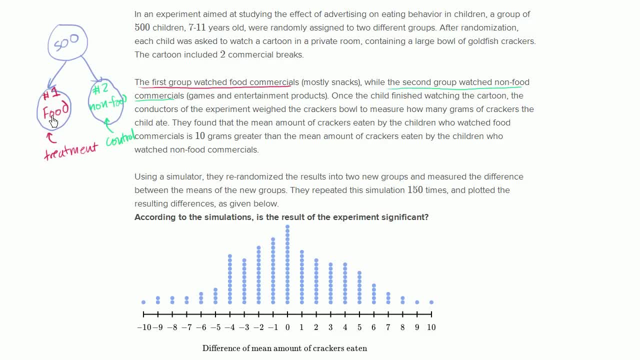 two random groups and you didn't make either group watch a commercial. you made them all watch the same commercials. there's some chance that the mean of one group could be dramatically different than the other one. It just happened to be So. number 2, this is the control group. 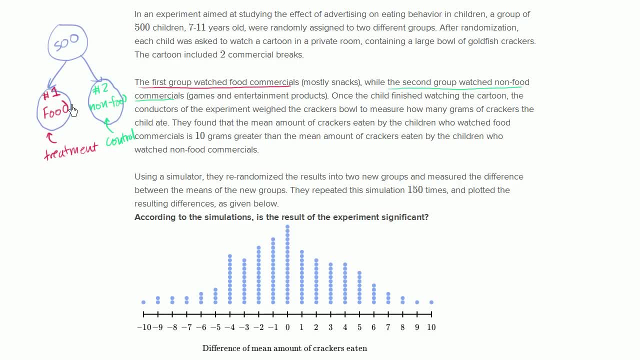 And it just happened to be in this experiment that the mean here that it looks like the kids ate 10 grams more. So how do you figure out what's the probability that this could have happened, that the 10 grams greater in mean amount eaten here, that that could have just 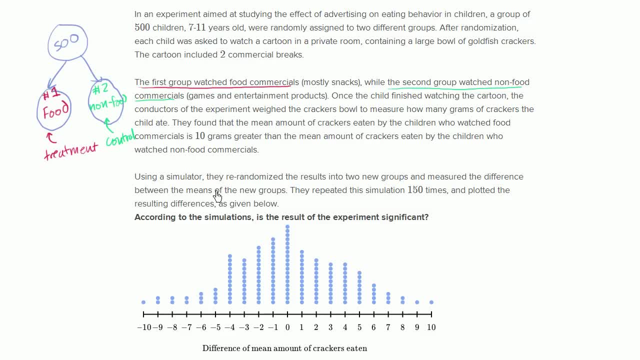 happened by chance. Well, the way you do it is what they do right over here. Using a simulator, they re-randomized the results into two new groups and measured the difference between the means of the new groups. They repeated the simulation 150 times. 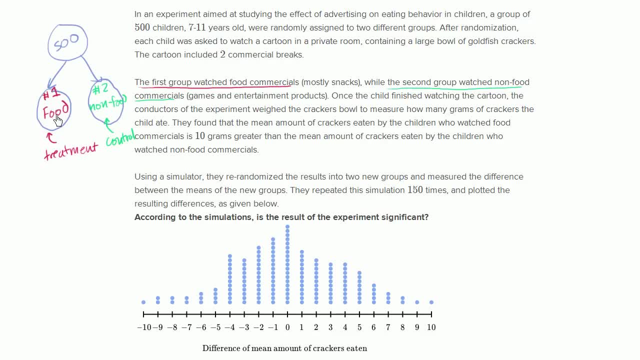 two random groups and you didn't make either group watch a commercial. You made them all watch the same commercials. There's some chance that the mean of one group could be dramatically different than the other one. It just happened to be in this experiment. 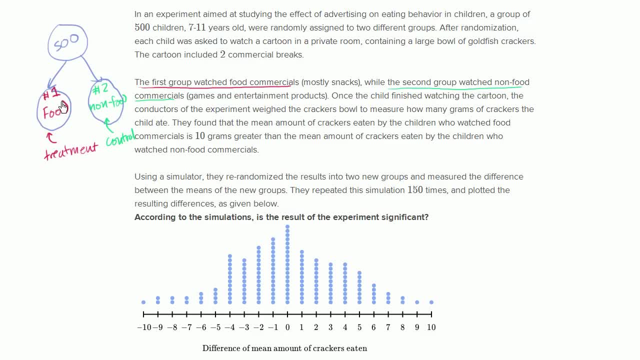 that the mean here that it looks like the kids ate 10 grams more. So how do you figure out what's the probability that this could have happened, that the 10 grams greater in mean amount eaten here, that that could have just happened by chance? 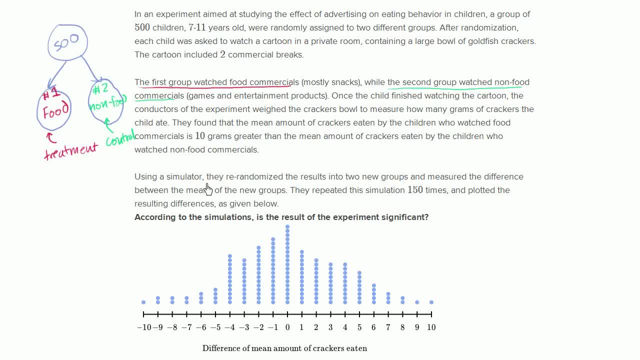 Well, the way you do, it is what they do right over here. Using a simulator, they re-randomized the results into two new groups and measured the difference between the means of the new groups. They repeated the simulation 150 times and plotted the resulting differences as given below. 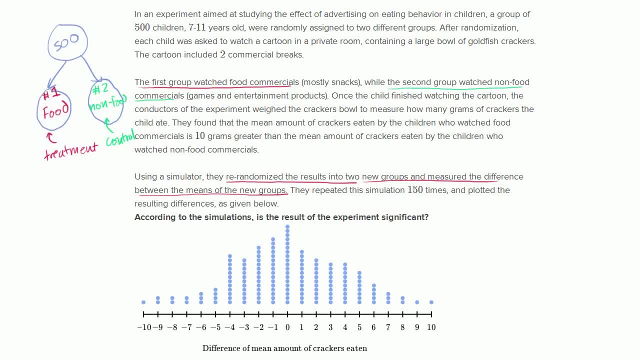 So what they did is they said, OK, they have 500 kids, And each kid they had 500 children. So number one, two, three, all the way up to 500. And for each child they measured how much was the weight of the crackers. 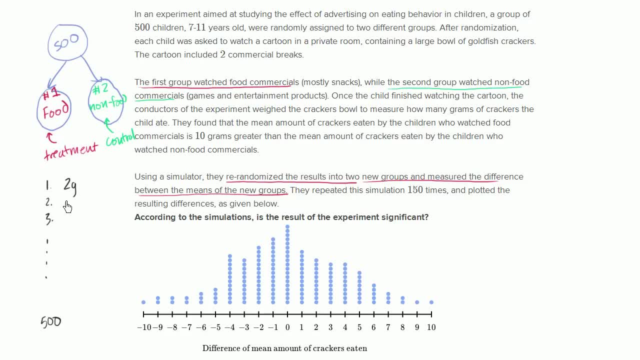 that they ate. So maybe child one ate 2 grams and child two ate 4 grams and child three ate- I don't know- ate 12 grams, all the way to child number 500, ate I don't know. maybe they didn't eat anything at all. 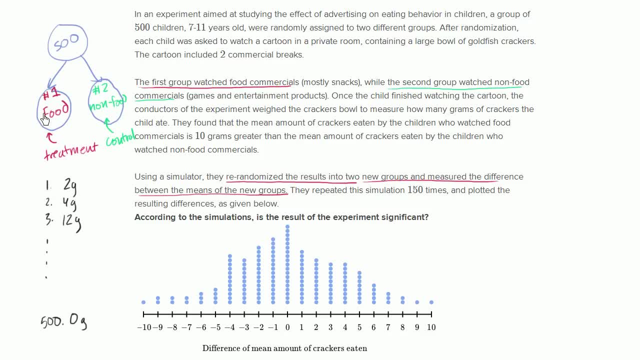 ate 0 grams And we already know, and let's say the first time around, one through 200 and one through, I guess we should. the first half was in the treatment group, when they were just ranking them like this, And then the second they were randomly assigned. 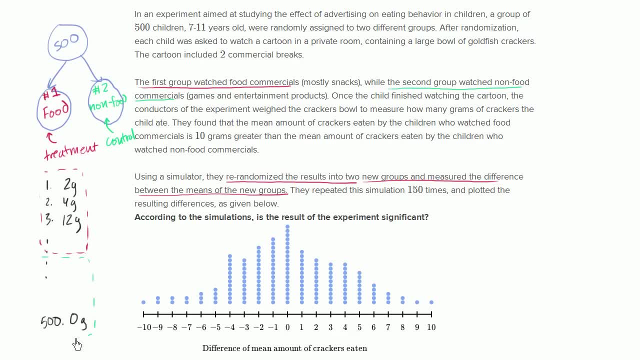 into these groups And then the second half was in the control group. But what they're doing now is they're taking these same results and they're re-randomizing it. So now they're saying, OK, let's maybe put this person in group number two and this person in group number two. 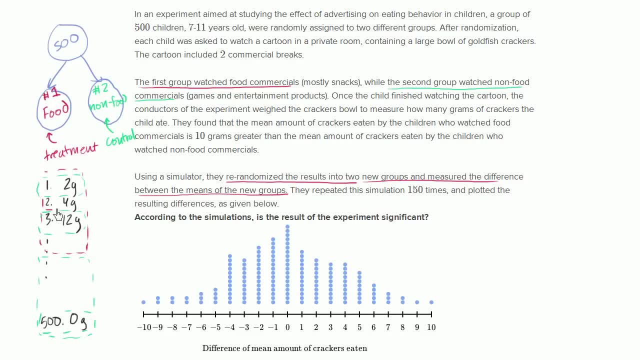 and this person stays in group number two and this person stays in group number one and this person stays in group number one. So now they're completely mixing up all of the results that they had. So it's completely random of whether the student had. 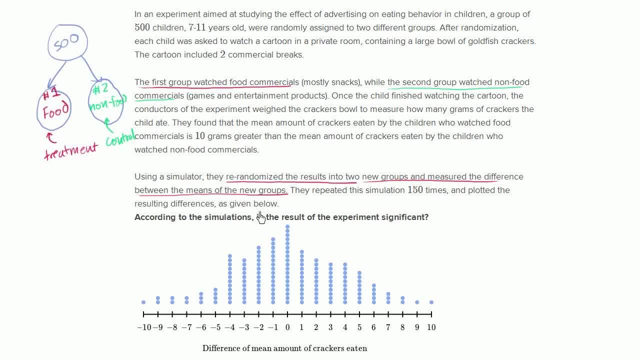 and plotted the resulting differences as given below. So what they did is they said: OK, they have 500 kids, And each kid they had 500 children. So number 1,, 2,, 3,, all the way up to 500. 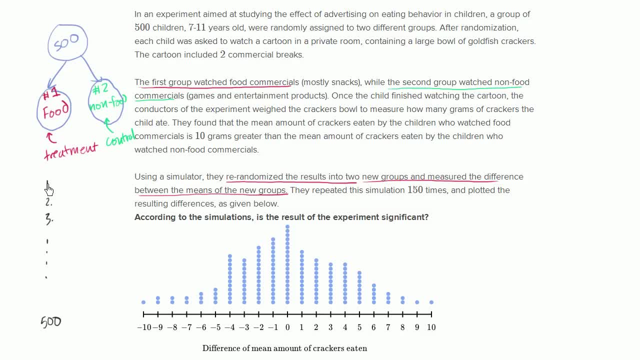 And for each child they measured how much was the weight of the crackers that they ate. So maybe child 1 ate 2 grams And child 2 ate 4 grams And child 3 ate- I don't know, ate 12 grams. 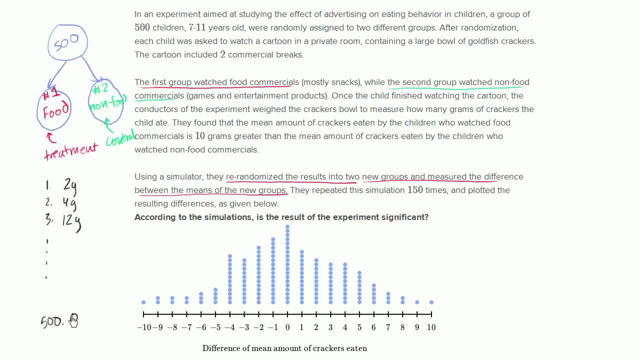 All the way to child number 500 ate. I don't know, maybe they didn't eat anything at all- ate 0 grams. And we already know, and let's say the first time around: 1 through 200 and 1 through. I guess we should. 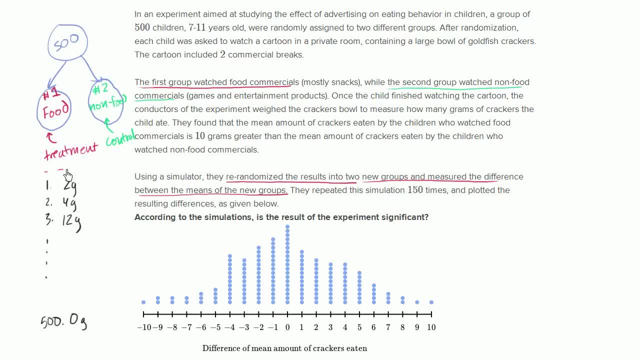 you know, the first half was in the treatment group when we were just ranking them like this, And then the second they were ranking them, They were randomly assigned into these groups And then the second half was in the control group. But what they're doing now is they're taking these same results. 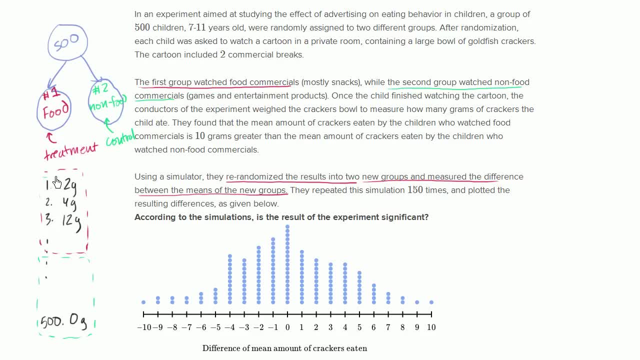 and they're re-randomizing it. So now they're saying, OK, let's maybe put this person in group number 2, and this person in group number 2, and this person stays in group number 2, and this person stays in group number 1,. 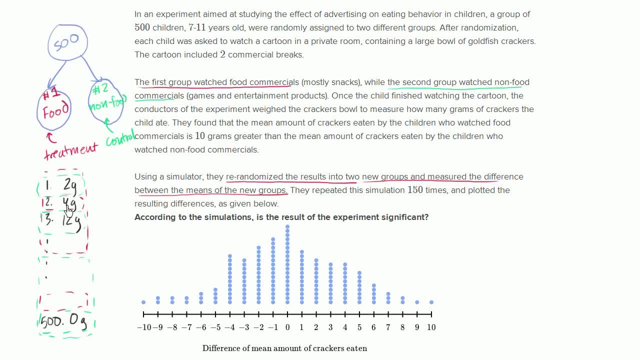 and this person stays in group number 1.. So now they're completely mixing up all of the results. So it's completely random of whether the student had watched the food commercial or the non-food commercial. And then they're testing what's the mean of the new number 1. 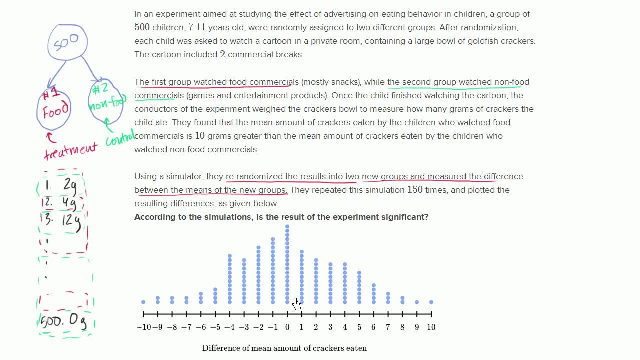 group and the new number 2 group. And then they're saying, well, what is the distribution of the differences in means? So they see, when they did it this way, when they're essentially just completely randomly taking these results and putting them into two new buckets. 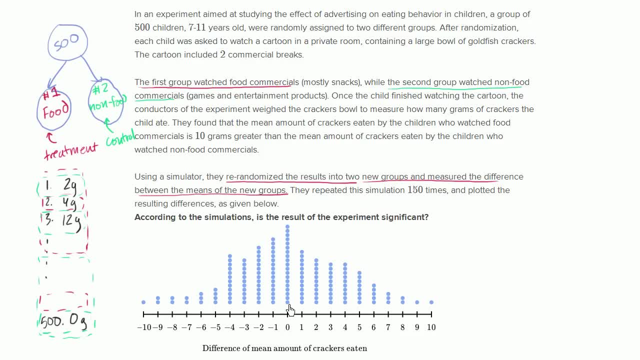 you have a bunch of cases where you get no difference in the mean. So out of the 100 cases you get 1.2.. So out of the 100 cases you get 1.2.. So out of the 100 cases you get 1.2.. 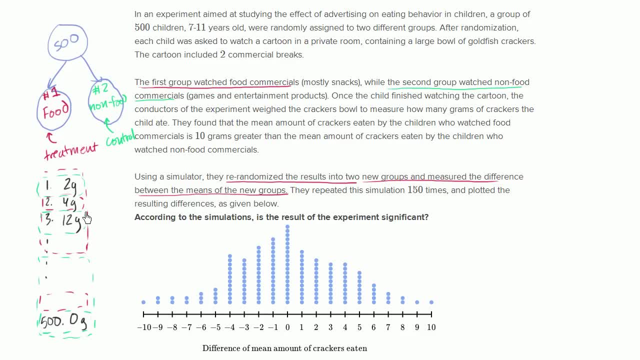 watched the food commercial or the non-food commercial, And then they're testing what's the mean of the new number one group and the new number two group? And then they're saying, well, what is the distribution of the differences in means? So they see, when they did it this way, 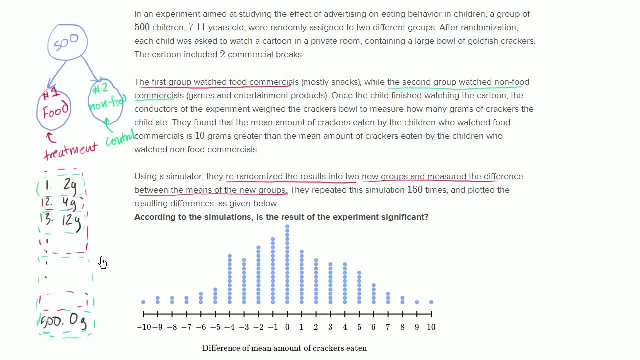 when they're essentially just completely randomly taking these results and putting them into two new buckets. you have a bunch of cases where you get no difference in the mean. So out of the 150 times that they repeated the simulation doing this little exercise here, 1, 2,, 3, 4,, 5,, 6,, 7,, 8,, 9,, 10,. 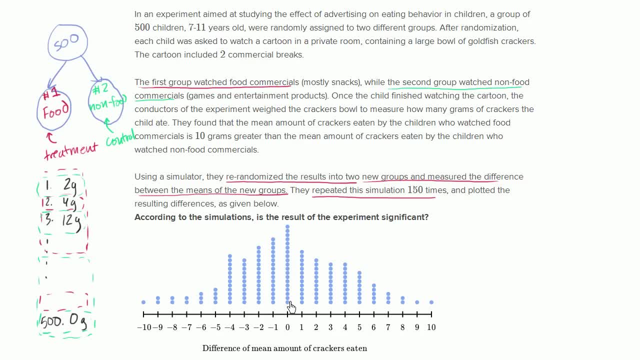 11,, 12,, 13,, 14,, 15,. I'm having trouble counting this. I see 1,, 2,, 3,, 4,, 5,, 6,, 7,, 8,, 9,, 10,, 11,, 12,. I keep it's so small. 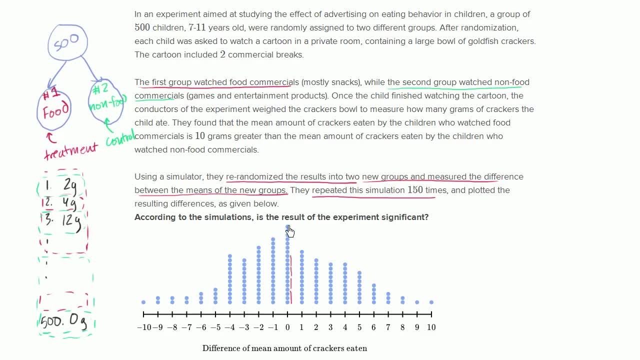 I'm aging, But it looks like there's about- I don't know- high teens. It's about 20 times when there was actually no noticeable difference in the means of the groups, where you just randomly allocate the results amongst the two groups. 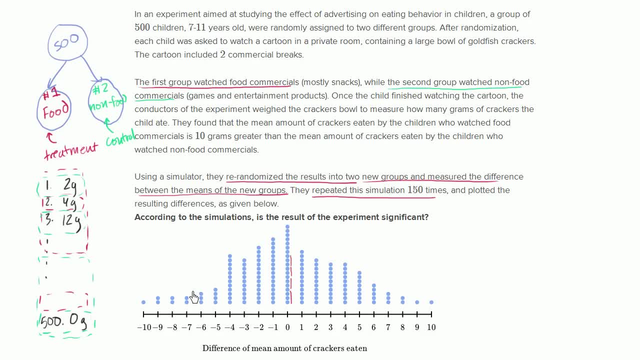 So when you look at this, if you just randomly put people into two groups, the probability or the situations where you get a 10-gram difference are actually very unlikely. So this is, let's see. is this the difference between the means of the new groups? 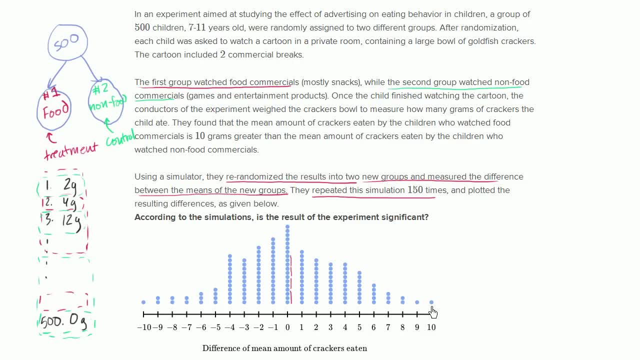 So it's not clear whether this is group 1 minus group 2 or group 2 minus group 1.. But in either case, the situations where you have a 10-gram difference in mean it's only 2 out of the 150 times. 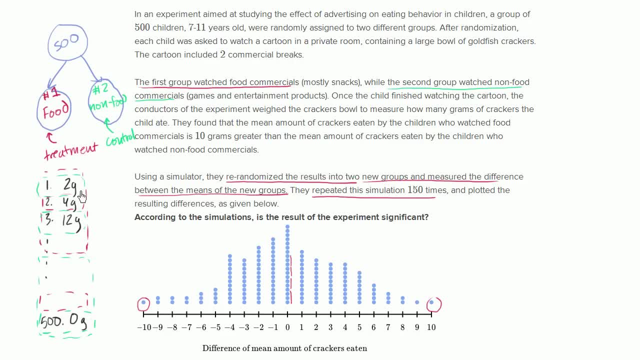 So when you do it randomly, when you just randomly put these results into two groups, the probability of the means being this different, it only happens 2 out of the 150 times. Yeah, OK, There's 150 dots here, So that is on the order of 2%. 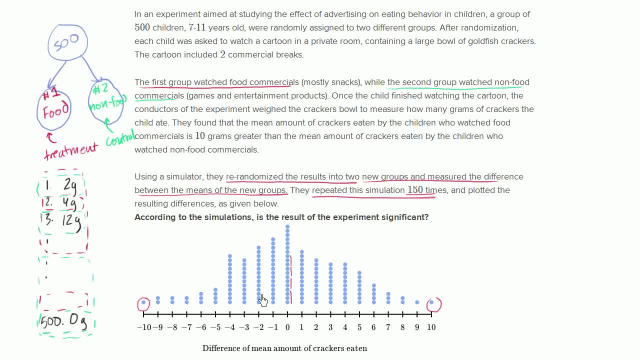 Or actually it's less than 2%. It's between 1 and 2% And if you know that this is group, let's say that the situation we're talking about, let's say that this is group 1 minus group 2 in terms. 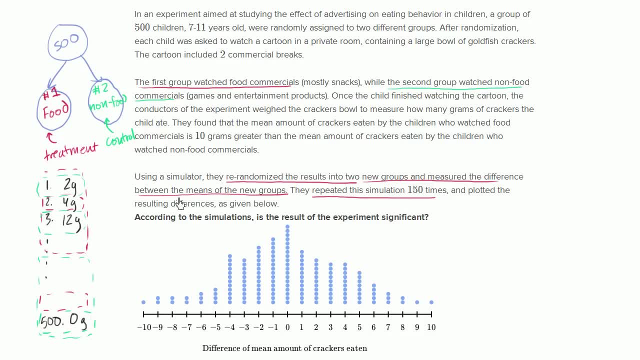 So out of the 100 cases, you get 1.2.. So out of the 150 times that they repeated the simulation doing this little exercise here, 1,, 2,, 3,, 4,, 5,, 6,, 7,, 8,, 9,, 10,, 11,, 12,, 13,, 14,, 15.. 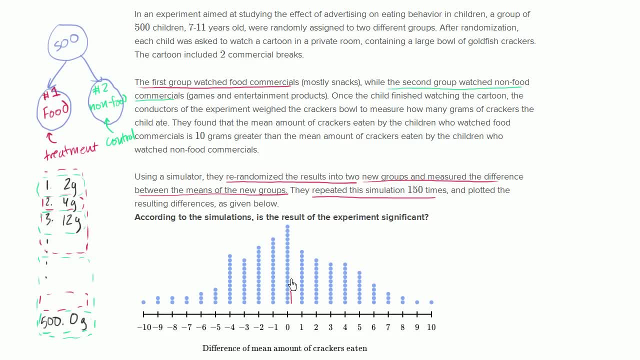 I'm having trouble counting this. I see 1,, 2,, 3,, 4,, 5,, 6,, 7,, 8,, 9,, 10,, 11, 12.. It's so small, I'm aging. 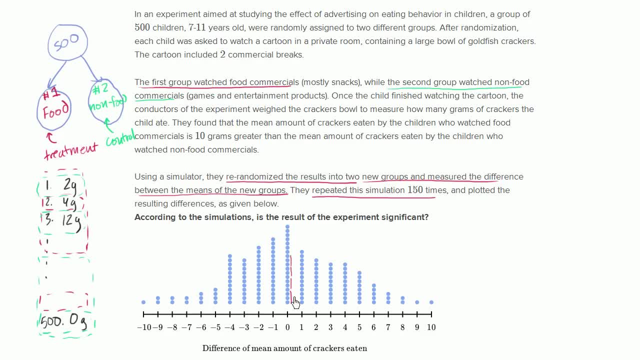 But it looks like there's about- I don't know- high teens- about 20 times. when there was one, there was actually no noticeable difference in the means of the groups when you just randomly allocate the results amongst the two groups. So when you look at this, if you just randomly put people 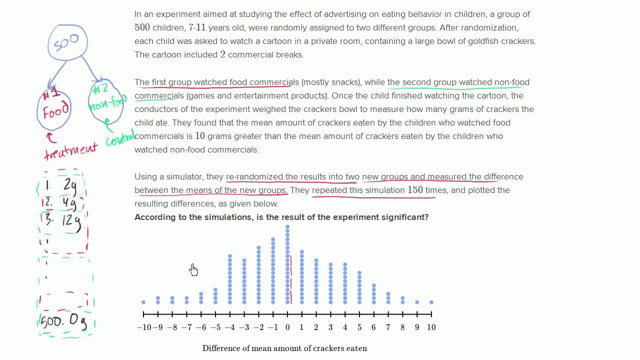 into two groups. the probability or the situations where you get a 10-gram difference are actually very unlikely. So this is, let's see. is this the difference between the means of the new groups? So it's not clear. It's not clear whether this is group 1 minus group 2. 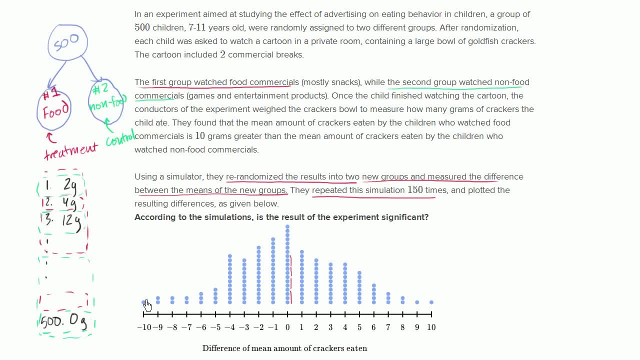 or group 2 minus group 1. But in either case the situations where you have a 10-gram difference in mean it's only 2 out of the 150 times. So when you do it randomly, when you just randomly, 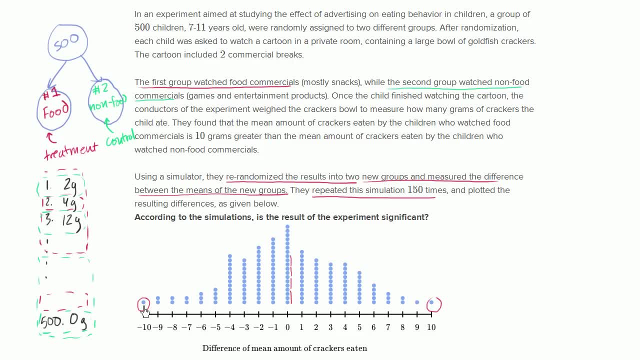 put these results into two groups, the probability of the means being this different. it only happens 2 out of the 150 times There's 150 dots here, So that is, It's on the order of 2%, Or actually it's less than 2%. 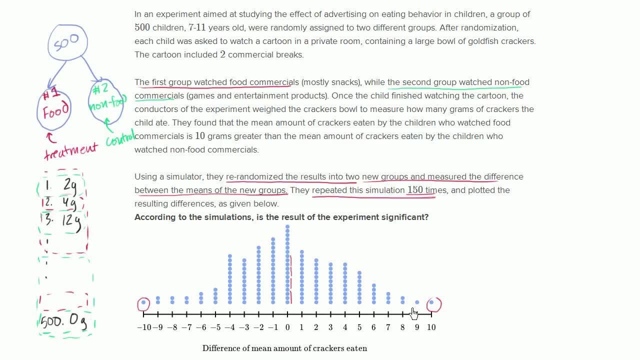 It's between 1 and 2%, And if you know that this is group, let's say that the situation we're talking about, let's say that this is group 1 minus group 2 in terms of how much was eaten, And so you're looking at this situation right over here. 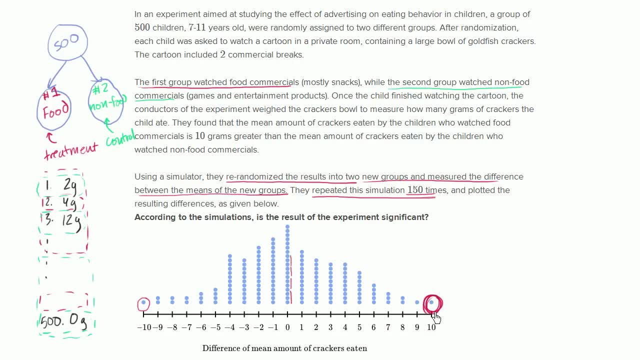 of how much was eaten, And so you're looking at this situation right over here. Then that's only 1 out of 150 times. So it happened less frequently than 1 in 100 times. It happened only 1 in 100 times. 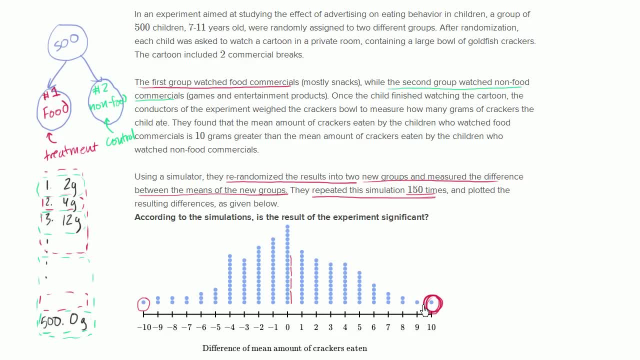 Then that's only 1 out of 150 times. So it happened less frequently than 1 in 100 times. It happened only 1 in 150 times. So if you look at that you say, wow, this was just random. 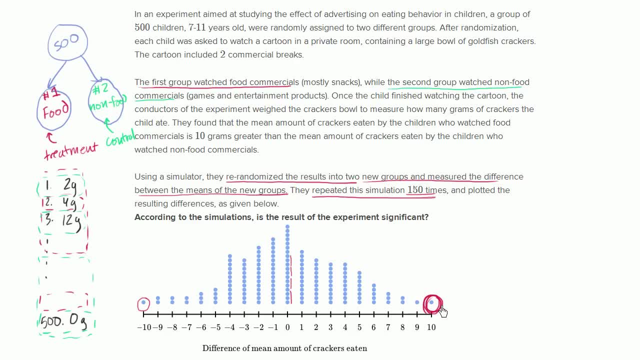 The probability of getting the results that you got is less than 1%. So to me, and then to most statisticians, that tells us that our experiment was significant, That the probability of getting the results that you got so the children who watched food commercials- being 10 grams. 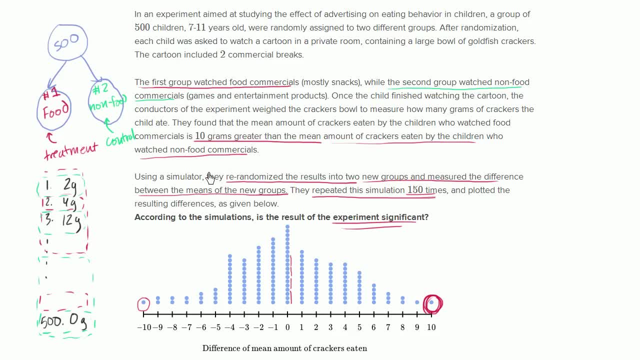 greater than the mean amount of crackers eaten by the children who watched non-food commercials. if you just randomly put 500 kids into two different buckets based on the simulation results, it looks like there's only out of you 2 out of 150 times.